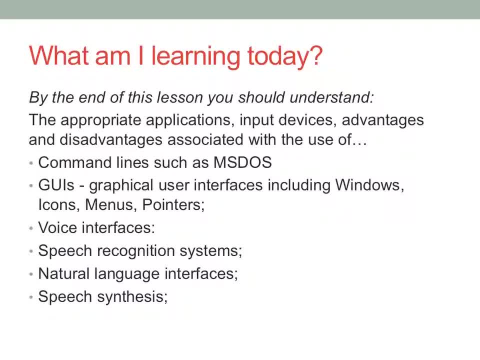 look at today will be command line interfaces like MS-DOS, graphical user interfaces like Windows or OS X, voice interfaces like when you speak to your phone, maybe speech recognition systems When they understand you, And natural language interfaces where they can actually interpret. 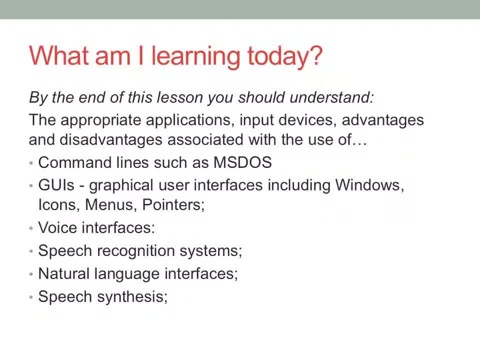 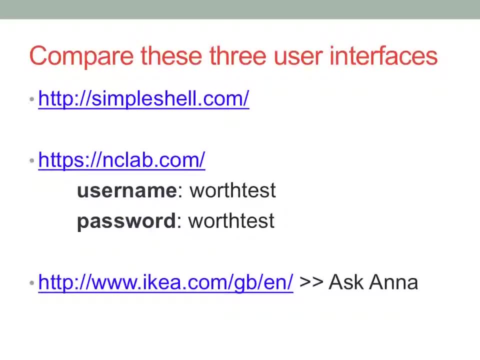 what you're saying. And finally, speech synthesis, where the machine will speak back to you. So lots of exciting things. The first step is a bit of a task. I'd like you to look at each of these websites in turn, Probably pause the video and then have a think about what sort of advantages and disadvantages. 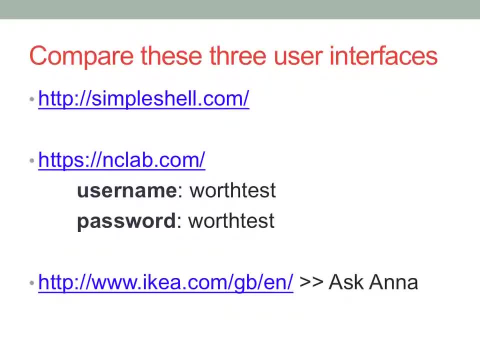 there are in each of these approaches to interface. They're all web-based tools, so you don't need to have any special software installed, And in the NC lab you can use the username worth test and the password worth test, or you can set up your own account And 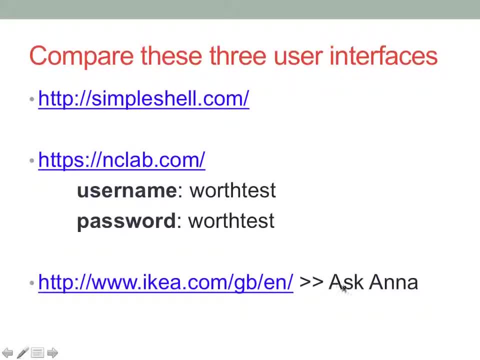 with the IKEA, you'll need to click ask Anna. and with the simple shell, you'll need to start the shell running. Okay, so I'll give you a minute to turn off. Okay, so, I'll give you a minute to turn off. 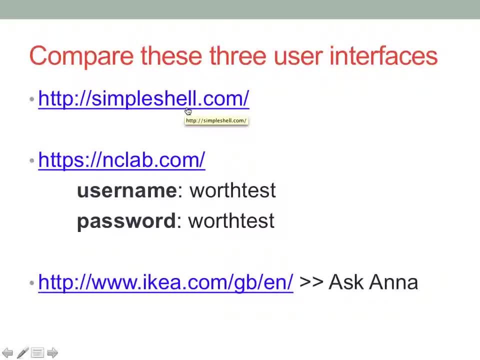 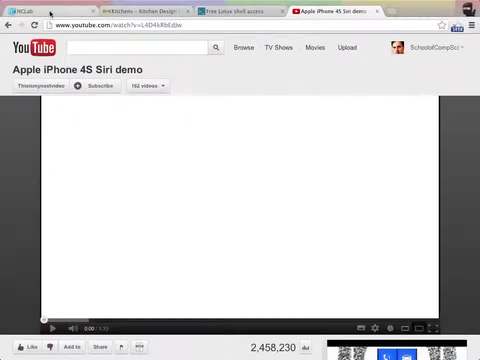 And then turn on again In a bit. So hopefully you're back now. after playing with them, We're going to go and have a look at them each individually in turn, So the first one I'm looking at is NC lab Now, despite being also a great place to learn. 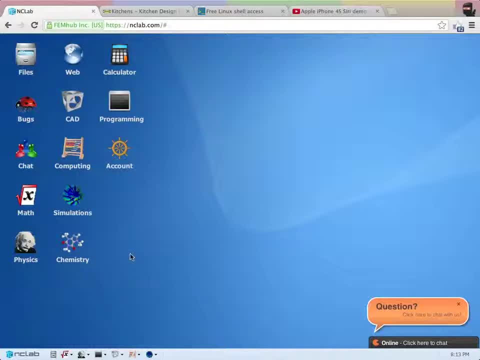 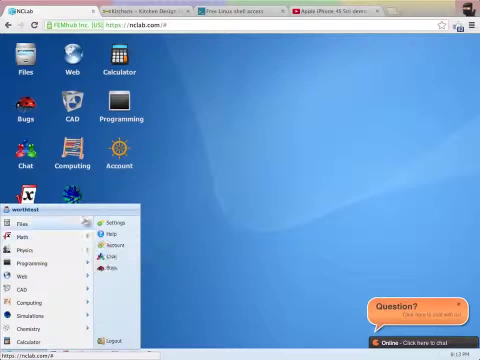 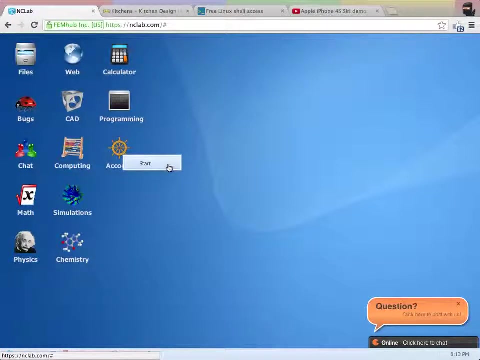 about computer science. NC lab represents essentially a graphical user interface in the way that there are menus when you click buttons And you've got a pointer, as in the cursor moving around your screen, your screen, you can right click on things to draw it, to drag out menus and and there are icons. 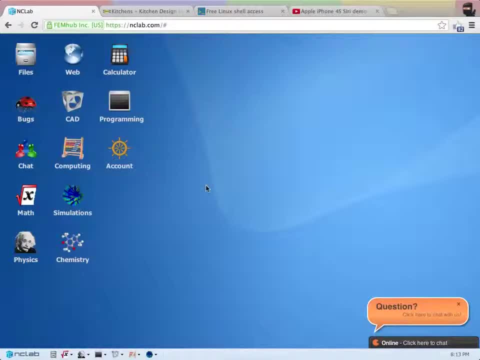 so those are windows icons, menus and pointers and and that's a a really uh intuitive interface and for people to use. it's really simple to learn how to use and unfortunately it does incur quite a lot of processing power and which is why some people might be using a another system which is called 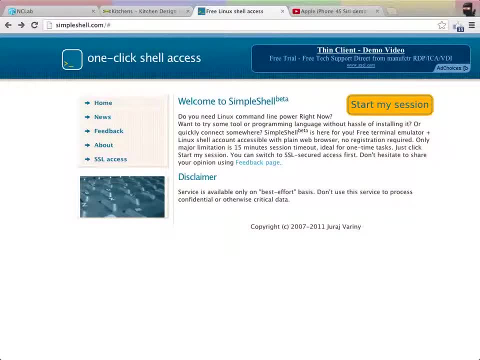 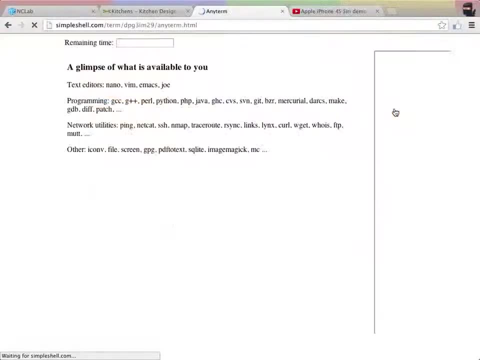 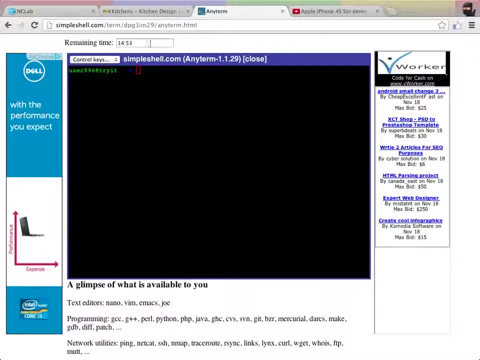 a command line interface, so when you go to the, the simple shell website, you can click start my session. this is a really nice um way to learn linux, which is an operating system, and, and in here this represents a command line interface. in fact, it represents the linux command line interface, and. 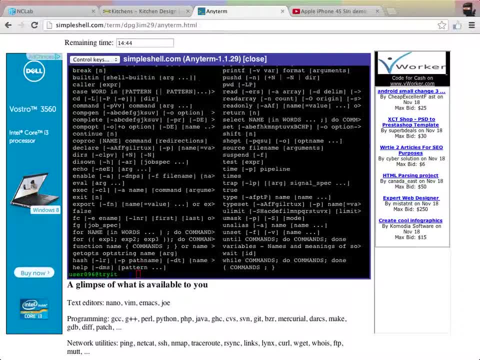 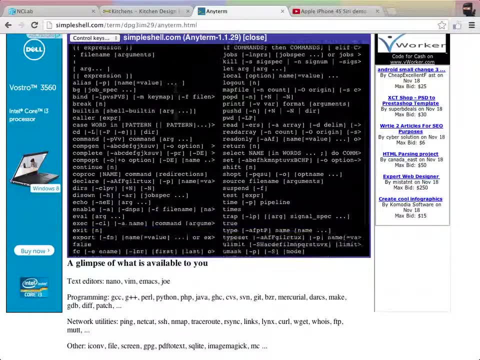 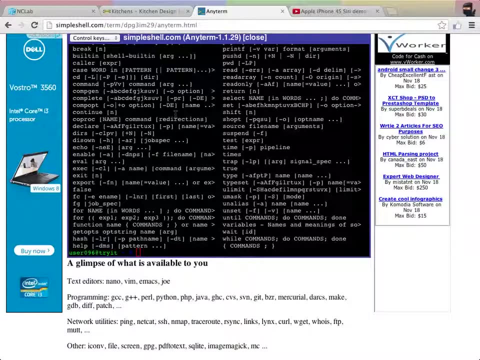 you can type in commands. so if i start off with help, it then lists a whole range of different um things that you can do, and the disadvantage of using an operating system like this is that you'll really to become any good at it, you need to actually remember all of the operations and um. 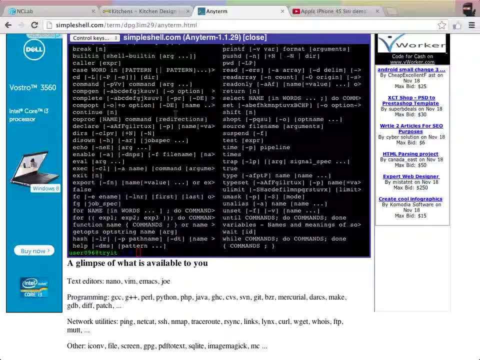 what they do and that can take a long time. however, it can be really powerful. some of the annoying operations, and with a graphical user interface, like when you want to change the setting on a range of files, can be done in a single line, in a command line interface, and that's why you find that. 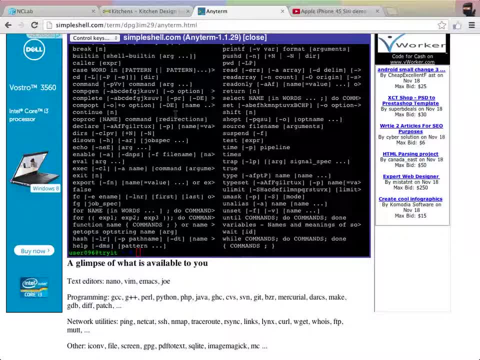 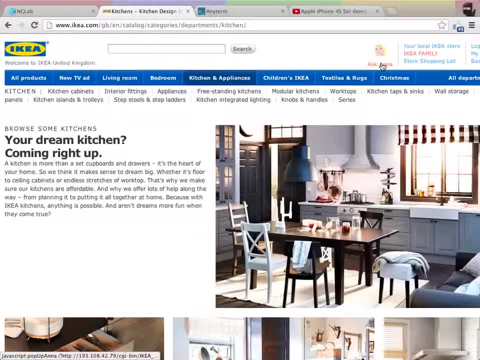 quite like using a command line interface. the next um approach i'd like you to look at is this: ask anna, which is found at the ikea home site. i think this is really interesting. so it's a um automated assistant, but actually it's a natural language processing system, so you can ask. 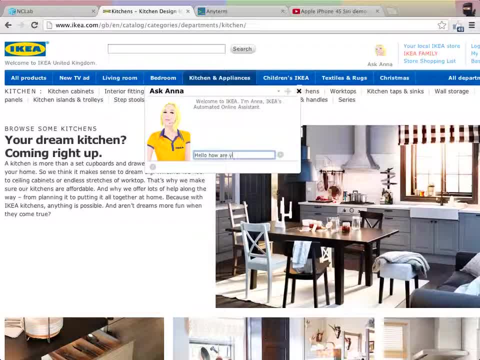 anna questions like hello, how are you doing? and you can expect her um to apply in an intelligent way. um, now, this info uses a form of artificial intelligence which processes natural language and also learns from conversations they've had in the past, and this is called heuristics, um, and it forms a much more kind of natural way of talking to someone, because 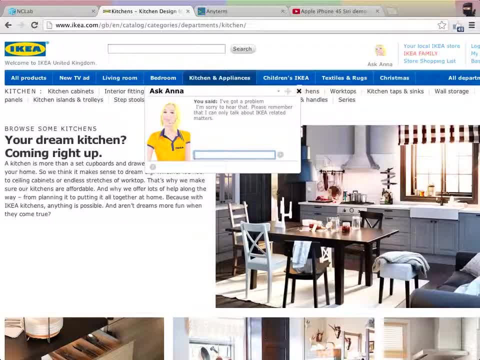 um, you can talk to them as if you're talking to another human, and there are limitations of the software and occasionally it gets things wrong, but i think this is a really good way to do that and this is a field of interface that will really, really improve in the future. another type: 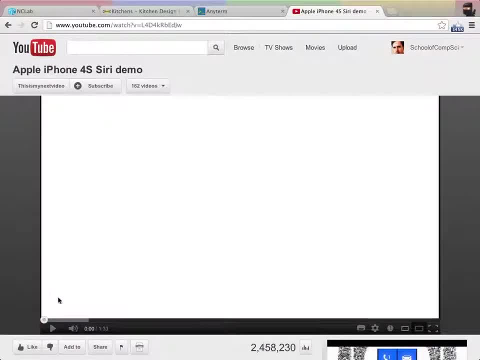 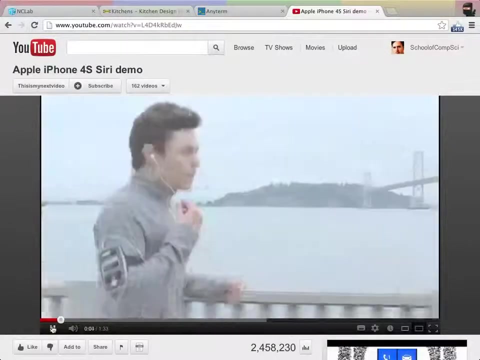 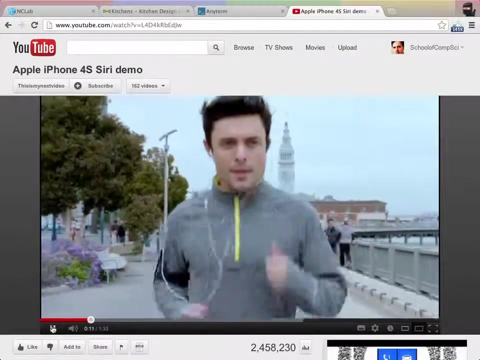 of interface you might be familiar with is the one that's being used on the apple um iphone 4s, which is called siri. um, i will attempt to play this and um get a recording of it. read me the message. new message from sebastian. great news: we got the go-ahead. can you meet him? ten reply, definitely, i'll see you there. 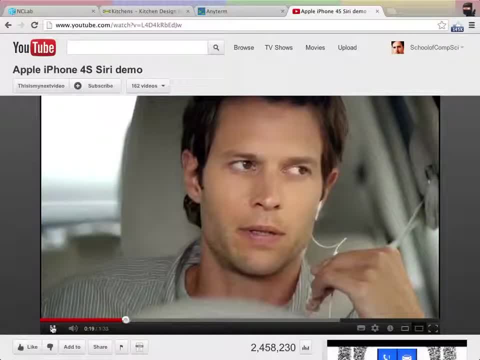 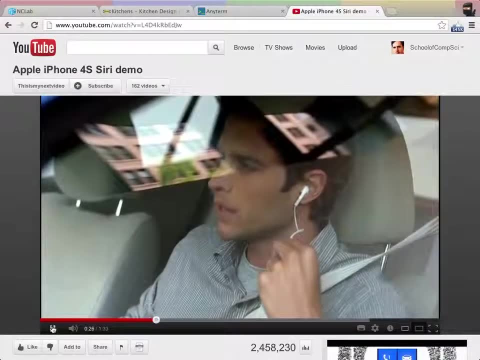 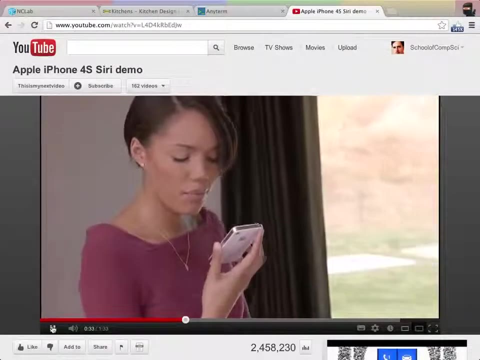 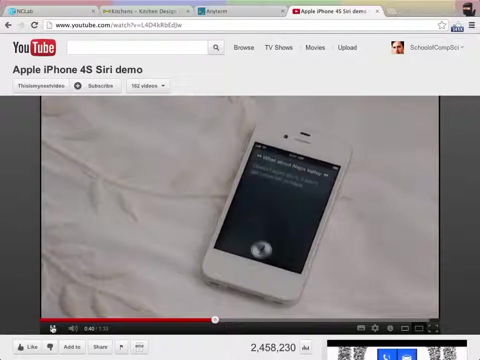 play my running mix. what's the traffic like around here? here's the traffic text. my wife- i'm gonna be 30 minutes late. is it going to be chilly in san francisco this weekend? not too long cold, maybe down to 61 degrees in san francisco. what about napa valley? doesn't seem like it. 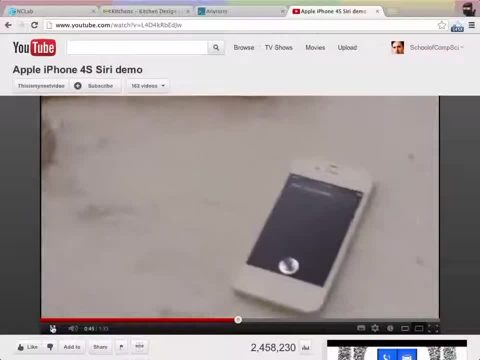 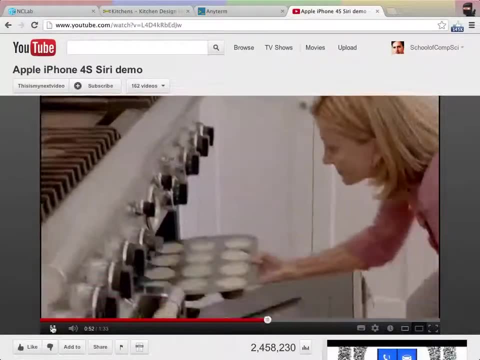 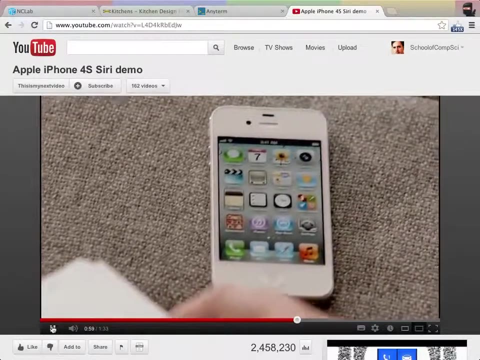 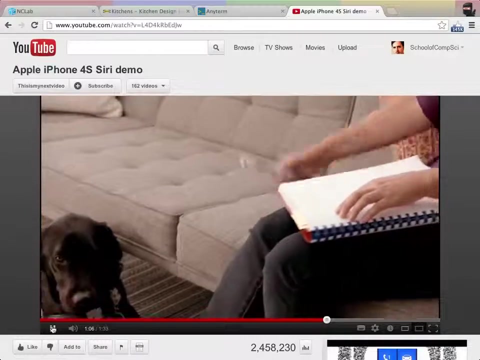 how many cups are in 12 ounces? let me think. okay, here you go. set my timer for 30 minutes. okay, 30 minutes and counting. new notification for messages. sandy jim, on four dinner tonight? reply. sure, i'll be there. here's your reply to sandy chen. 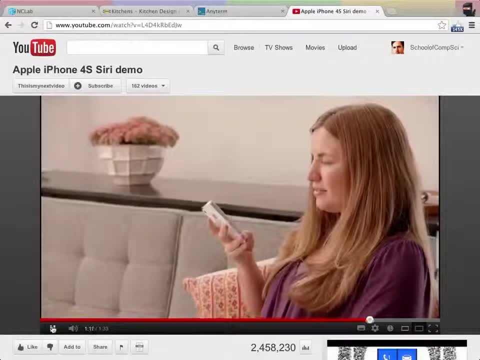 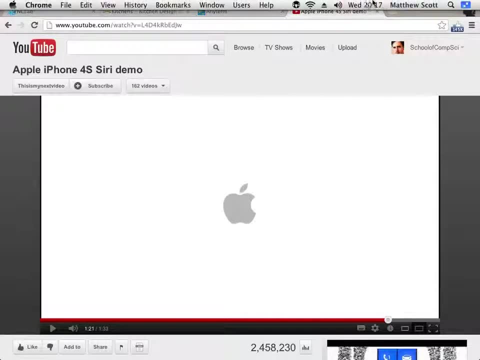 sure i'll be there. so within this system, we saw a range of different user interfaces and we saw speech recognition, where it could convert natural language, ничего language, into something the computer understands. We saw natural language processing, where the computer would then listen to what has been said and try and interpret the meaning behind. 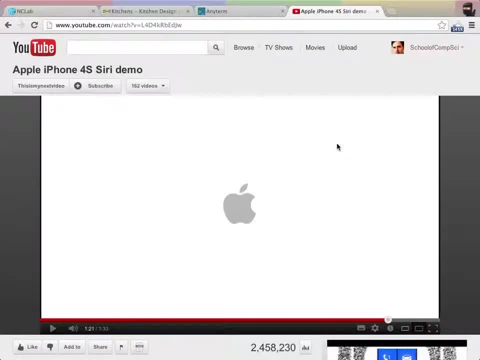 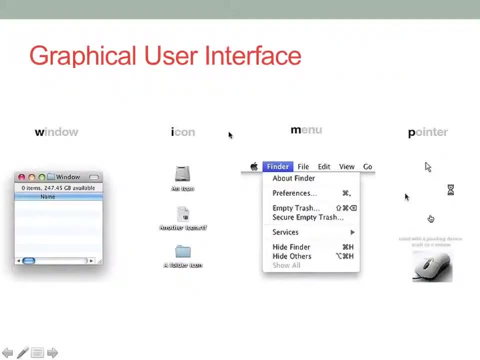 it. And then, finally, we saw voice output, where the computer would synthesise a human voice and speak back to us. So if we look at these different types of interface in a little bit more detail now, So we've got the graphical user interface which was seen in the NC labs. 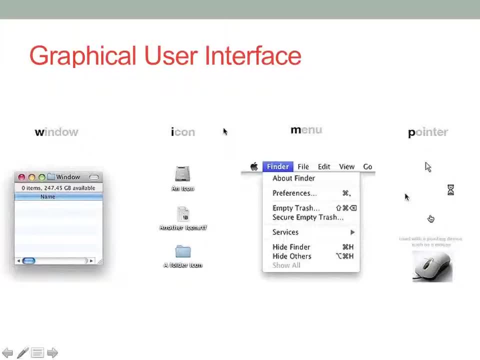 It's also what you'll be familiar with when you're using a desktop PC or a laptop, where you've got windows icons, menus and pointers. These have been around a long time. The input device required for them is a mouse and they're meant to form a very intuitive, natural way. 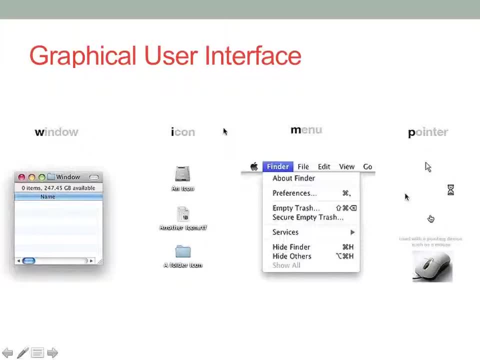 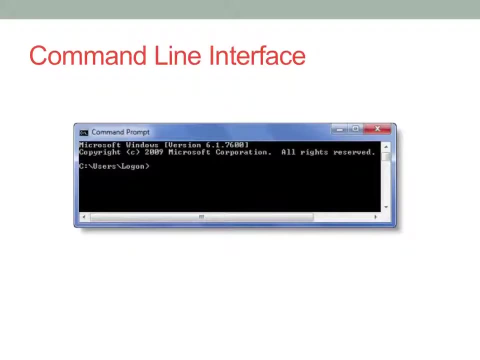 of manipulating data and files on a computer. The second one that we saw was the command line interface. Now, this doesn't require as much processing as a graphical user interface, and it can actually be quicker to perform commands on a range of different files in a single text entry. The downside: 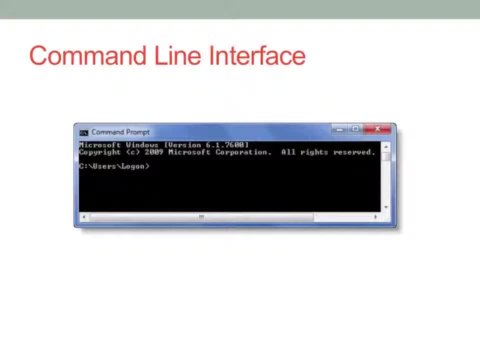 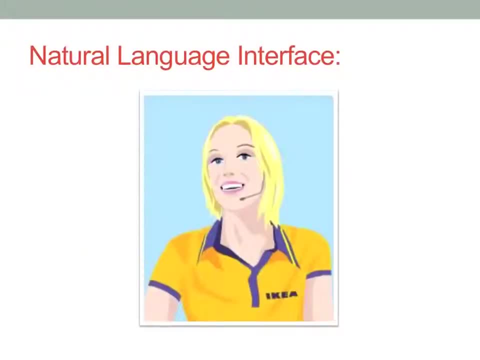 is that you have to memorise every single command and you need to be a real expert in order to use these. Then we went on and looked at the natural language interface which was provided by the Ikea Annie. We were able to have to have a kind of a chat conversation, and this is a 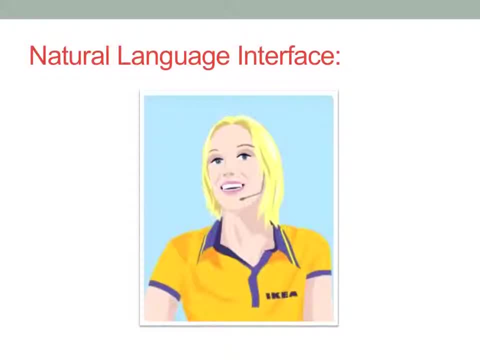 form of artificial intelligence. In fact, a famous computer scientist called Alan Turin defined a test for artificial intelligence whereby a computer could be called intelligent if a human didn't know that they were having a conversation with a computer through a chat interface. The advantages of this are that it's really intuitive for a human to use, because people 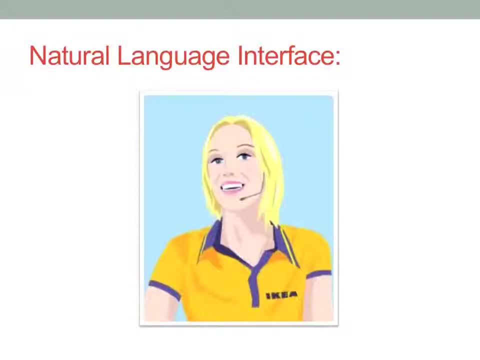 prefer to communicate in natural language, not points and clicks. The disadvantage is it's not really appropriate for handling files, for example, and also that it requires quite a lot of pre-programming. but an advantage of that is that it can learn over time. so 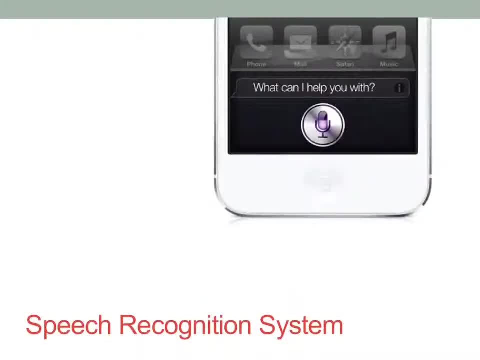 it can engage in machine learning. Finally, one of the examples we looked at was the speech recognition system. This is where speech is converted into text that a machine like the Ascani could understand, and the example we looked at was Siri, whereby you would say: 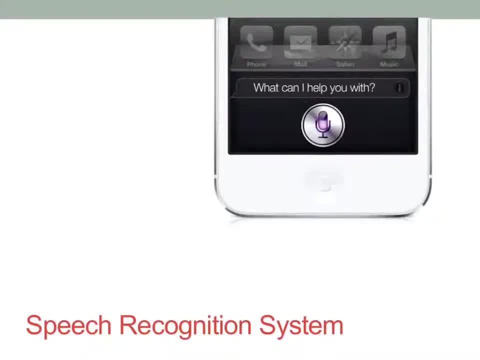 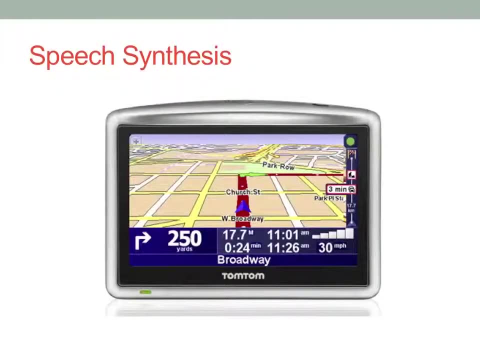 something and then Siri would recognise the words that you were saying. And another aspect of Siri was getting the computer to talk back to you, and you'll probably be. if you don't have an iPhone, you may well have a GPS system in your car. one of the screens are TomTom. 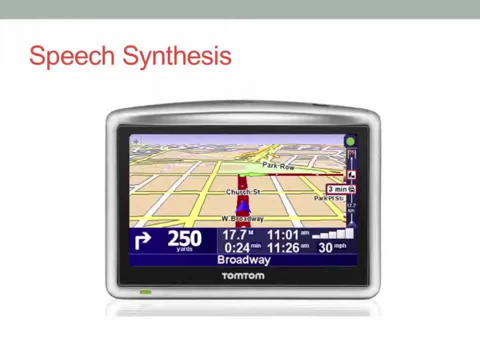 and they're probably the first mainstream application to use this. There was a thing called Microsoft Mary, which was used to read what was on the screen on Windows machines. However, I think that this is more sort of widely adopted, and the reason why TomTom uses a voice output is because when you're 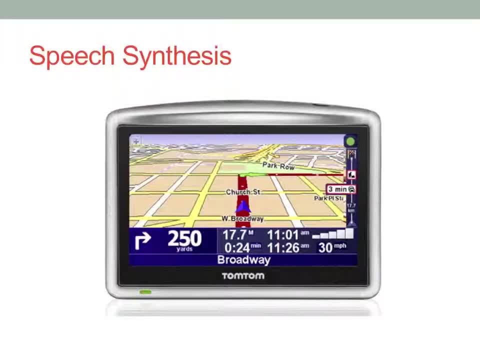 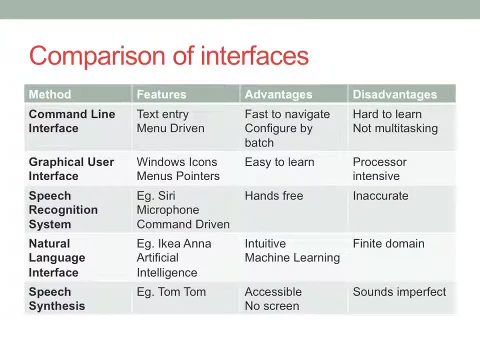 driving, you can't actually be looking at the screen all the time because you've got other things to do, and so it was a very sensible choice for TomTom to have voice output. So the table here summates the advantages, disadvantages and applications of all these. 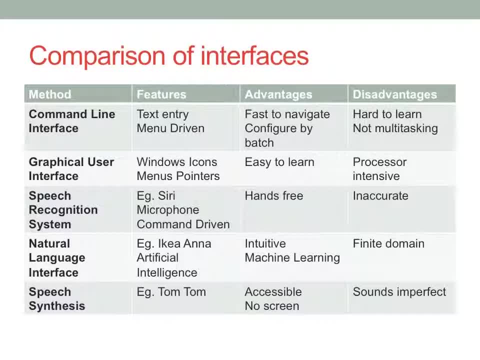 different interfaces. We've got a command line interface which is where you type in commands. There is an option where you'd have a menu-driven interface which is slightly more usable within a command line interface. So in text you'd be given options like press 1 to do this, press 2 to 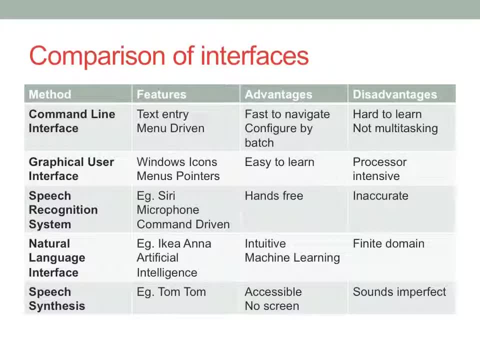 do this. press 3 to do this. If you've used a very old cache machine, it would be it actually used a system like this. The advantages of a command line interface is it's actually really fast to jump between files And you can configure the settings on a file by batch in a very short bit of by typing: 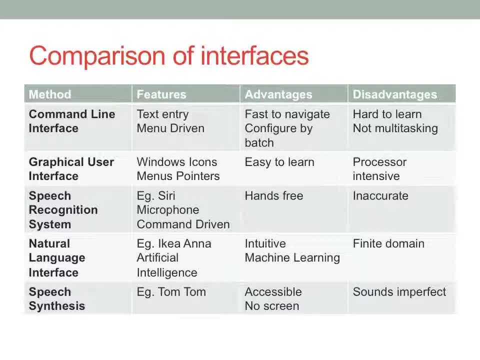 in a very short statement or command. The disadvantage is it's really hard to learn and many of the command line interface operating systems don't do multitasking. So in a Windows operating system where you can have more than one window open at once and jump between programs, it's actually not as common in a command line. 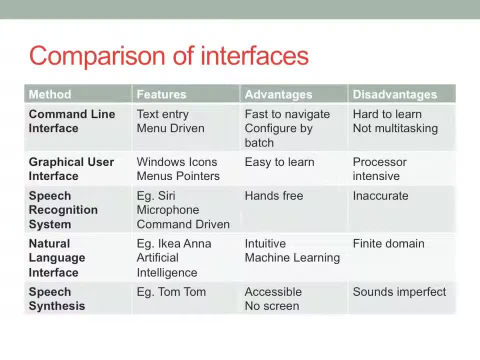 interface for that to happen. The next section was the graphical user interface. The next section was the graphical user interface. The next section was the graphical user interface. This was the thing that used Windows icons, menus and pointers and used on many desktop. 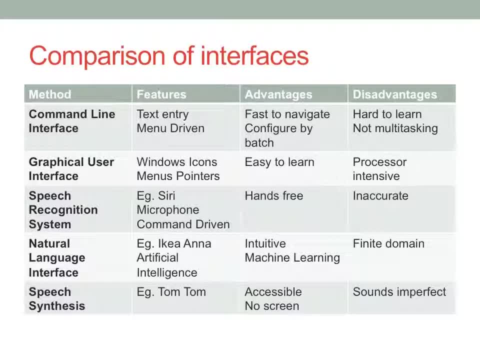 PCs, both Apple and Windows alike. I suppose the key advantage is it's very easy to learn, but the disadvantage is that it's processor intensive. Moving on, you had speech recognition systems, and the most common form of speech recognition that I've seen at the moment is the Siri. The input device required for that is a microphone. 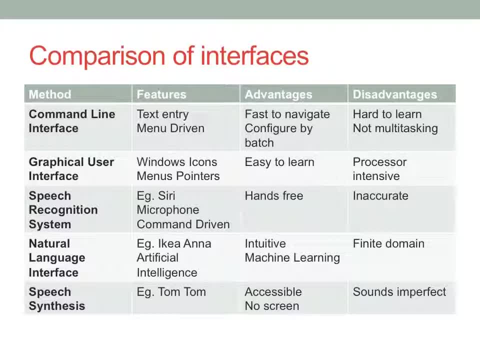 and it can be quite command-driven. so it won't. it's not until you apply a natural language interface that it actually starts to interpret what you say. The advantages of it is that it's hands-free, so you can control the computer without actually having to either look at. 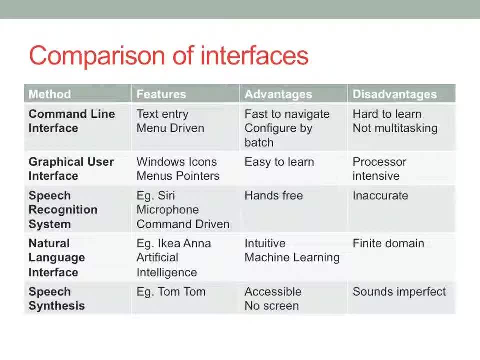 a screen or use a mouse. The disadvantage is it's quite inaccurate and requires some for you to train the speech recognition software. The next thing that we've looked at is natural language interfaces. A good example of this is the Ikea Ask Anna. This employs and converts text into command-driven speech recognition. 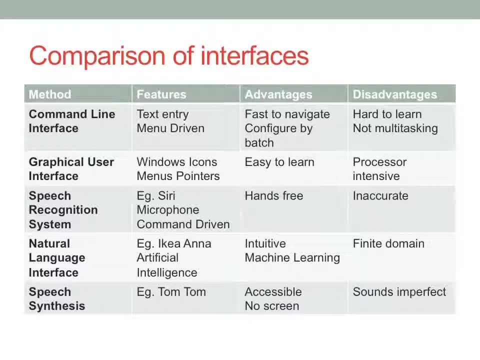 The Ikea Ask, Anna will look up the correct response from a database of responses that have been successful in the past. This is known as a heuristic and it's a form of artificial intelligence. It's really intuitive. As I said, it uses machine learning and it's great. 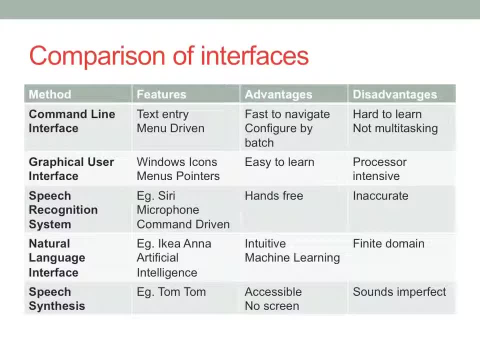 in customer service applications. The disadvantage is that really Ask Anna has quite a finite domain. She's only really intelligent about things that are to do with Ikea. If you ask her the meaning to life and everything, I doubt that she'll have a sufficient answer. 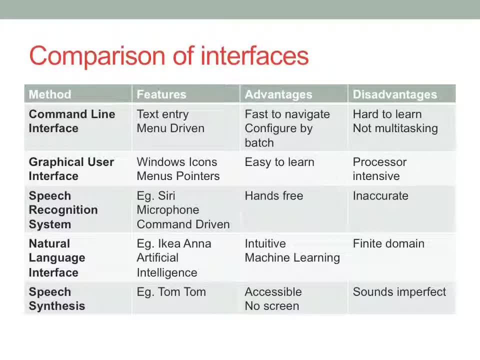 And then, finally, we've got the speech synthesis, which just requires a computer and a speaker, and a good example of which is TomTom for the satellite navigation system. It's really accessible, so people who are blind, who can't see the screen, could be using it, And also. 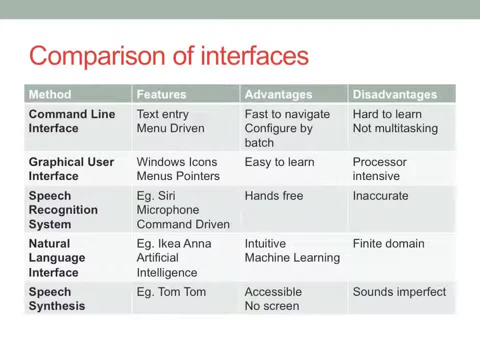 it's very good for when you've got your attention on something else and so you don't have a screen to look at. However, the sound does sound a bit creepy, and so it's not quite perfect. human speech. 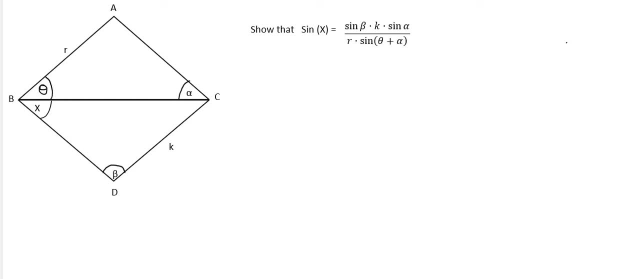 Hello everyone, welcome to this lesson. In this lesson, we're going to be looking at the type of questions where they don't give you any numbers, but instead they give you letters. Now, a lot of students find this section quite confusing, but what I'm going to show you in this lesson is that 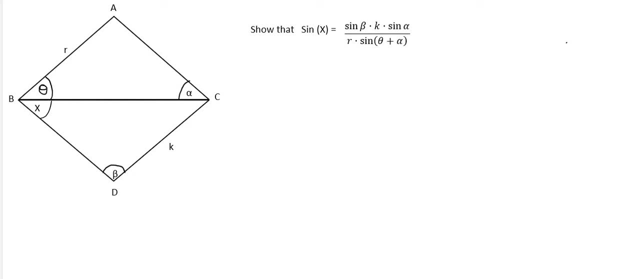 there is a pattern that you can follow when solving these types of questions. So what you've got to do is you've got to look at the question first of all. So the question wants us to eventually find the sin of angle x. Okay, now x is over here in this bottom triangle, So what? 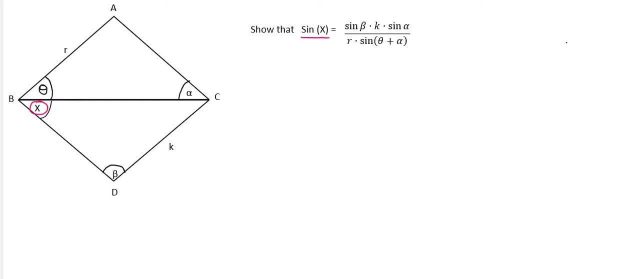 you're typically going to do is: don't work in that triangle just yet. You're going to work in the other triangle, So you're going to work in the top triangle first. Which side do you think we should find? Well, we eventually want to end up working in the bottom triangle, So what we're going to do